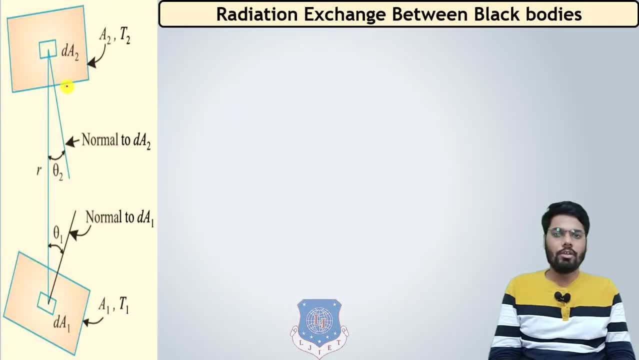 Suppose we have two bodies as shown in figure. The area of this plate is A1, which is maintained at temperature T1.. The area of second plate is A2 and temperature is T2 respectively. Now to derive the relation between heat transfer by radiation between these two plates, we have to consider the differential area of both the plates. 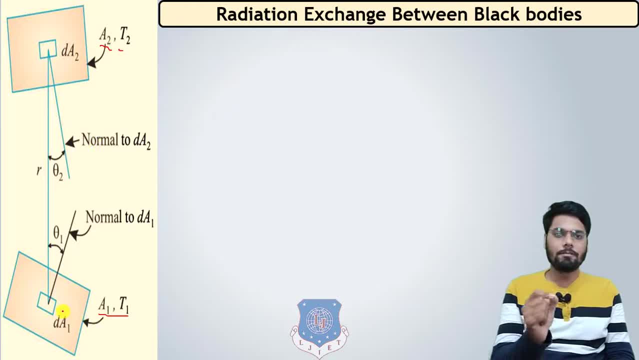 So for plate A1, we have considered small differential area, which is A1. Similar for plate A2.. The differential area which is considered is A2.. The distance between connecting the centre of both plate A1 and plate A2 is small, r, which is shown in figure. 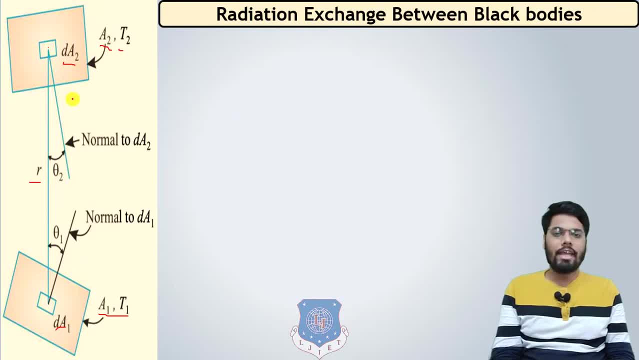 Now, from our knowledge of solid angle, we can say that d omega 1, which is solid angle, made by plate A2 and which is subtended at plate A1.. I repeat again: d omega 1 is a solid angle which is made by plate A2.. 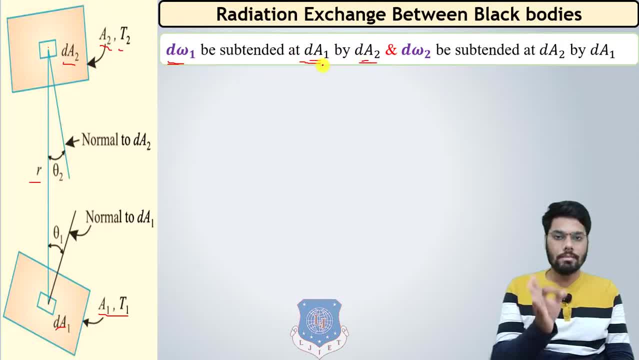 And which is subtended at diet A1.. Similarly, d omega 2 is the solid angle which is made by flint A1 and which is subtended at flint A2.. So, from the definition of the solid angle, we can write down: d omega 1 is equal to-. 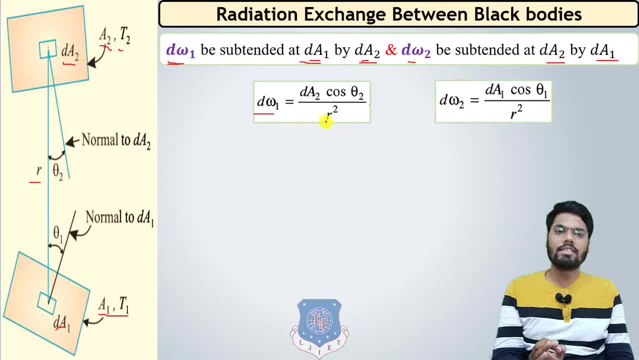 dimensions of flint A1 and d. omega 2 is r squared. Similarly, for a angle d, omega 2 is equal to flint A1 cos theta 2.. dA1 cos theta1 divided by r square. Now let's discuss about the energy leaving dA1 in the 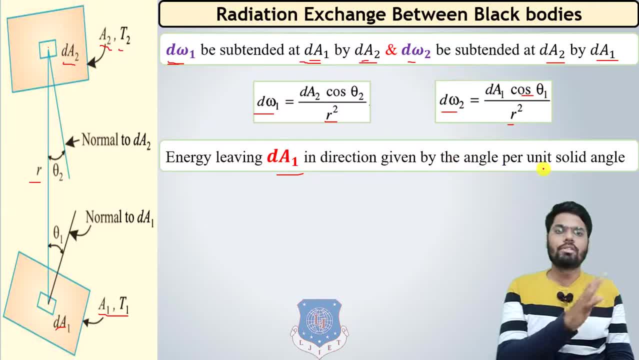 direction given by angle per unit solid angle. It can be written as: Ib1, dA1 cos theta1.. Here Ib1 is the intensity of black body and dA1 cos theta1 is for the direction. So Ib1 is black. 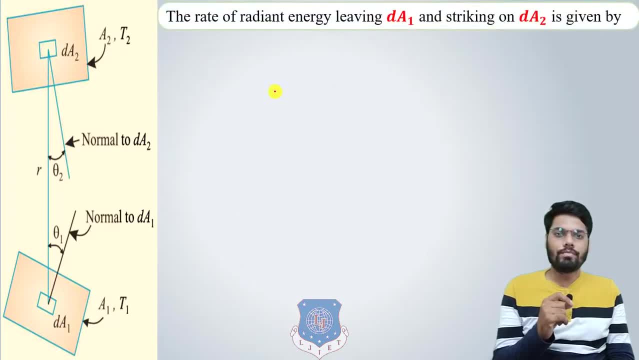 body angles. Now the rate of radiant energy leaving dA1 and striking on dA2 is given by dq1 to 122.. Here dq because the area which we have considered is a differential area, not the whole area, a1 and a2. It is about dA1 and dA2.. So the heat transfer between this dA1. 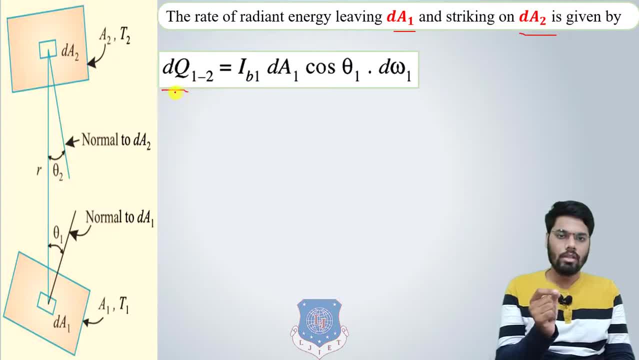 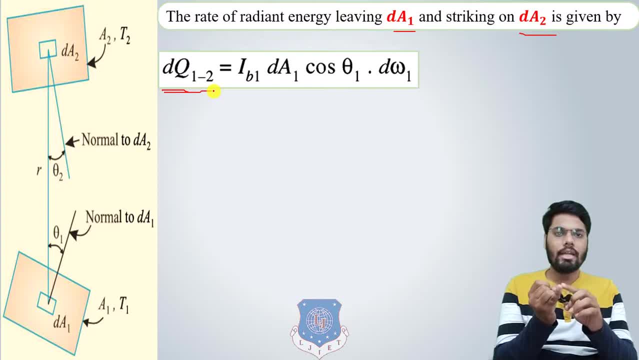 So this dq1 to 122 can be noted by dq1 to 122. This dq1 to 122 can be noted by dq1 to 122 means the energy or the electromagnetic wave which is emitting from dA1 and striking on dA2. that is given by Ib1, dA1, cos, theta1.. This is the amount of electromagnetic wave which is. 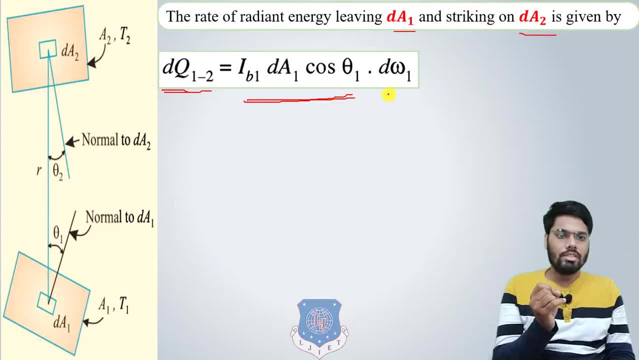 emission by dA1.. Now into the solid angle d, omega 1, because not all the electromagnetic wave which is emitted from dA1 is going to strike on dA2.. So here, both these db1 and db2, because of the orientation, there are some amount of electromagnetic wave which is emitted. 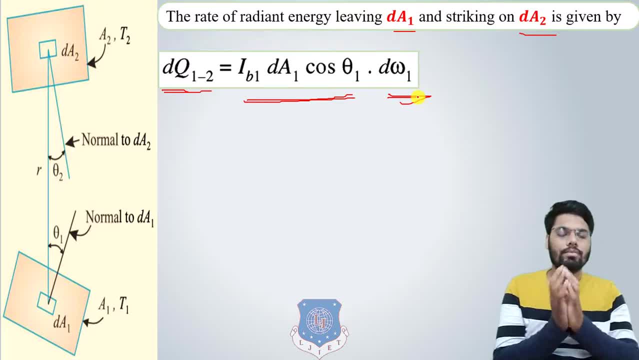 from the dA1 are going to incident on dA2, which is based on orientation and the solid angle made between dA1 and dA2. so the amount, or we can say that the radiant energy which is leaving the dA1 and striking dA2 is given by Ib1, dA1, cos, theta1, A2, d, omega1. now we know. 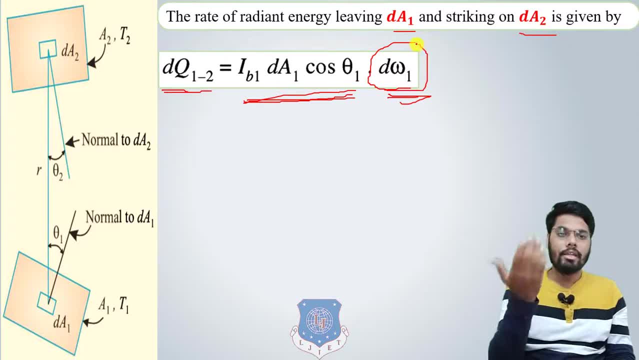 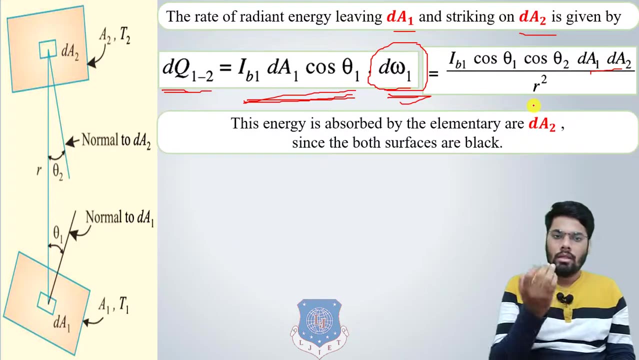 the equation for d omega1, the solid angle which is made by dA2, substandard to dA1. so by putting the value of d omega1, we will get Ib1 cos, theta1 cos, theta2, dA1, dA2 divided by R square. this energy is absorbed by the elementary R area, dA2, since the both surface. 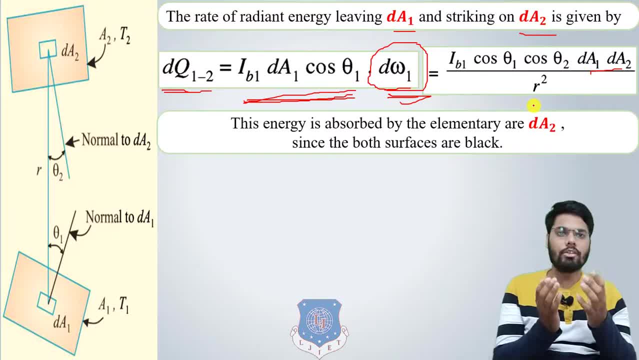 are black, so black surface absorb all the electromagnetic wave which is going to incident on it, Since all the energy is going to be absorbed by the area dA2. now the quantity of energy radiant by dA2 and absorbed by dA1 can, similarly given by Ib2 cos. theta2, cos, theta1, dA2, dA1. 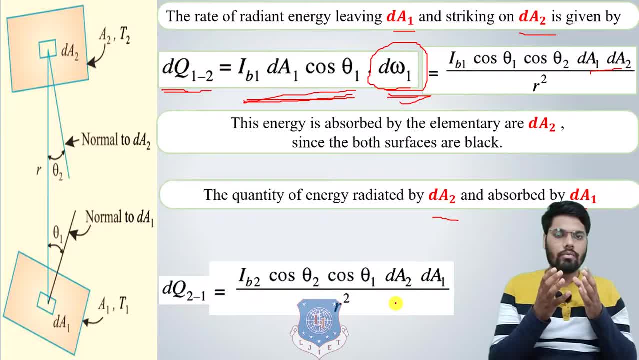 divided by R square, because in conduction beam whenever there is a temperature difference it will do system. the heat will flow from higher temperature system to the lower temperature system. similarly, in convection also the heat will transfer from the higher temperature system to the lower temperature system, but in a radiation if there are two plates: one. 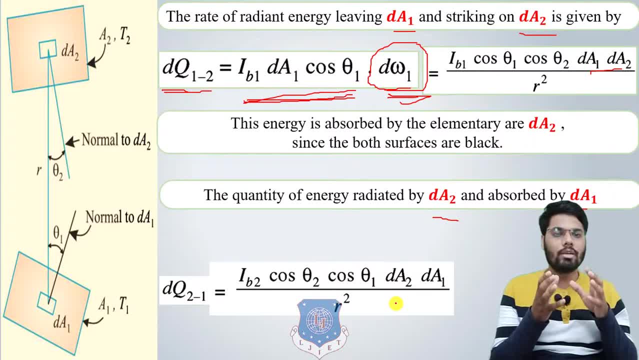 at temperature T1 and one at temperature T2. it doesn't matter whether T1 is greater than T2 or T2 is greater than T1. both the surfaces emit electromagnetic wave which is going to be incident on another surface. so here we have two plates: the differential area dA1. 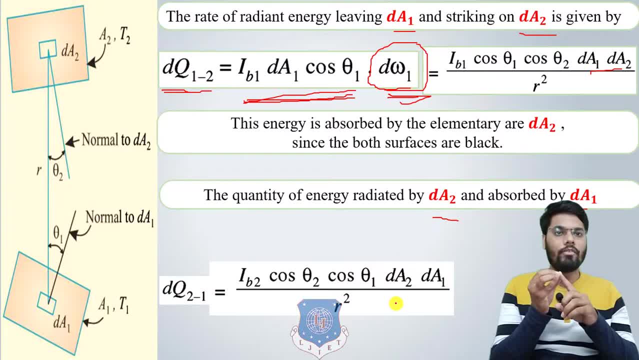 and dA2. so as we have considered that the some amount of electromagnetic wave which is going to be incident on another surface, so here we have two plates: the differential area dA1 and incident on another surface. so here we have some amount of electromagnetic wave. 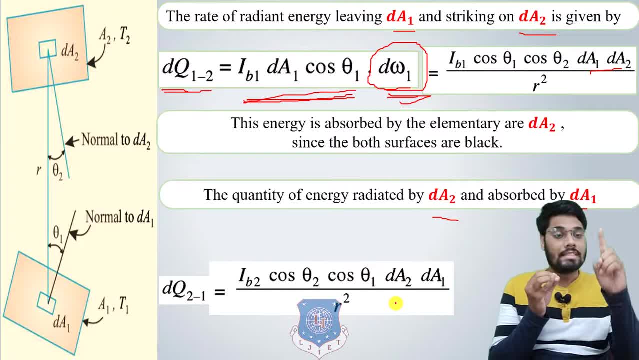 which is going to be emitted from the dA1 and incident on dA2. similarly, there are some amount of electromagnetic wave which is going to be emitted by dA2 and incident on dA1. so as we have written for equation for dq122, we can similarly write for dq221 is equal. 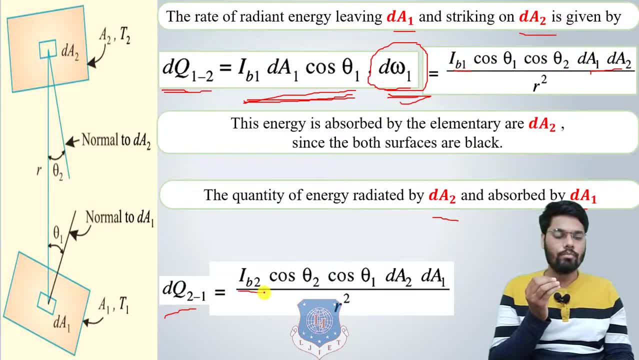 to. instead of Ib1. here it will be. it will be Ib2 cos, theta2 cos, theta1, dA2, dA1 divided by R square. so this is the current that we can write for the dq221. so this is our result for dQ222, and so this is the current that we can write for the dQ221. so this is the current. 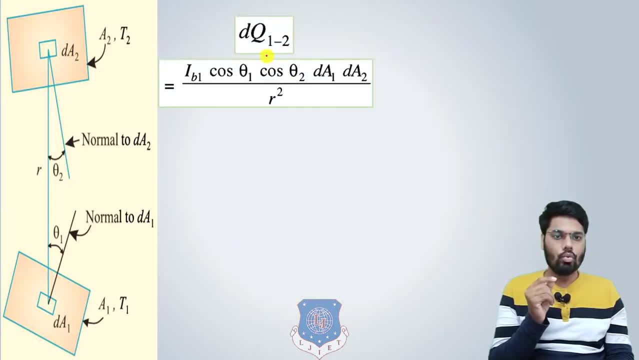 So we have equation for D2 1 to 2 and equation for D2 2 to 1.. This equation shows the amount of electromagnetic wave emitted from surface 1 and incident on 2.. This equation shows the electromagnetic wave emitted from surface 2 and incident on surface. 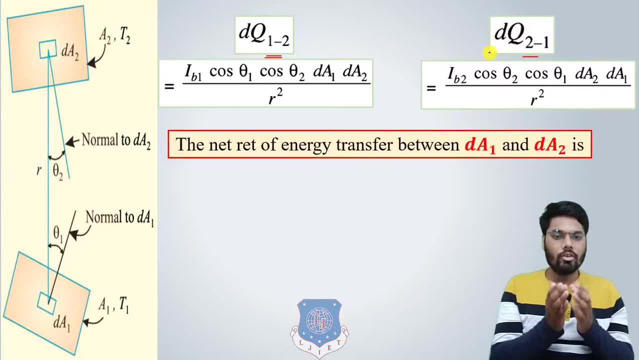 1. So from these two equations we can calculate the net rate of energy transfer between DA1 and DA2.. Suppose there are 10 kJ which is emitted from surface 1 and received by surface 2 and 3 kJ which is emitted by surface 2 and received by surface 1, then we can easily calculate. 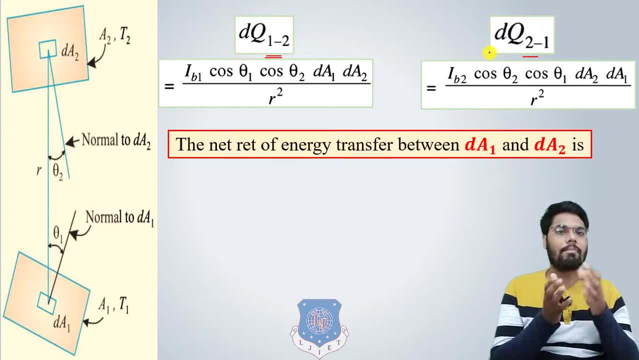 the net radiant heat transfer between these two surfaces by 10 minus 2.. So, similarly, DQ 1 to 2 is equal to DQ 1 to 2 minus DQ 2 to 1.. This DQ 1 to 2 represents the net heat transfer between these two surfaces by 10 minus 2.. 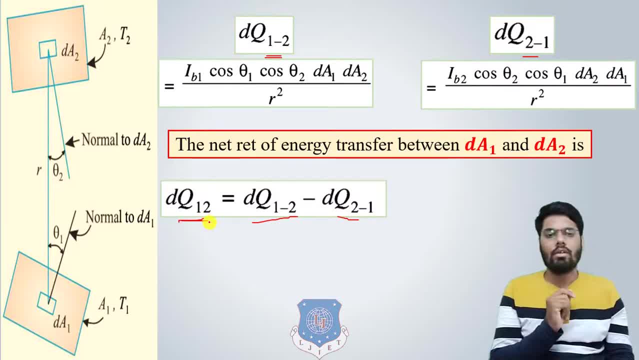 This net heat of the surface 1 to 2 is equal to DQ 1 to 2 minus DQ 2 to 1.. So when putting the value of this DQ 1 to 2 and DQ 2 to 1 here, cosθ1, cosθ2,, DA1,. 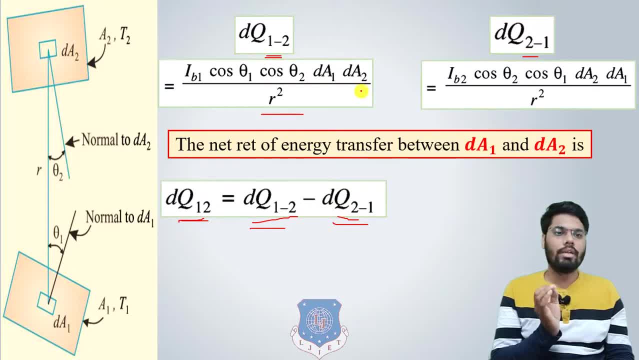 DA2 divided by R square will common in bracket. it is IB1 and IB2.. Now in this equation, IB1 and IB2 represent intensity of blackbody of surface 1 and surface 2 respectively. Now we know the relation of intensity and emissive power. in our previous video we have 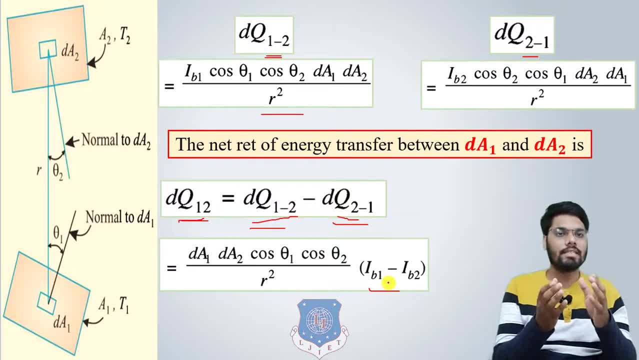 derived the relation between these two, So we are going to convert these two. the intensity of the radiation, which is intensity I, is equal to invasive power divided by pi. So for surface 1, IB1 is equal to EB1 divided by pi, and for surface 2, IB2 is equal to EB2. 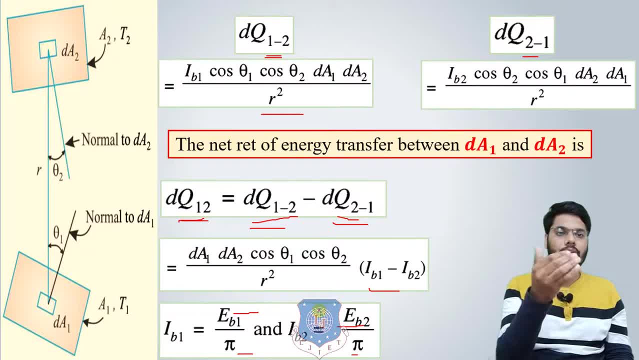 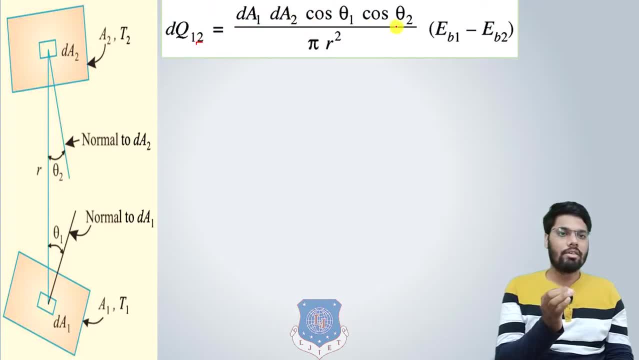 divided by pi. So putting the value of this IB1 and IB2 in our equation, we will get q. dq12 is equal to dA1, dA2 cos theta1, cos theta2 divided by pi. r square in bracket EB1 minus EB2.. 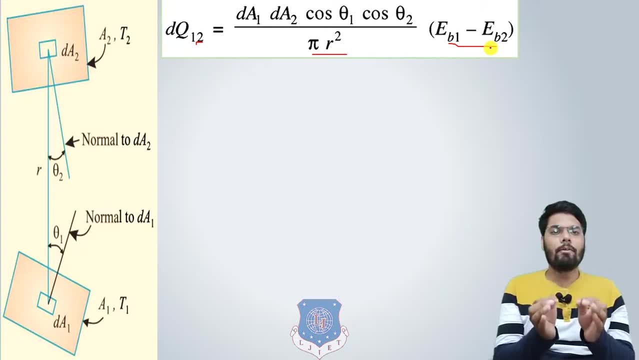 Now, in this equation, EB1 and EB2 is invasive power of black body. So from Stephen Boltzmann law, instead of EB1, we can write down sigma into T1, raise to 4, and instead of EB2, we can write sigma into T2, raise to 4.. 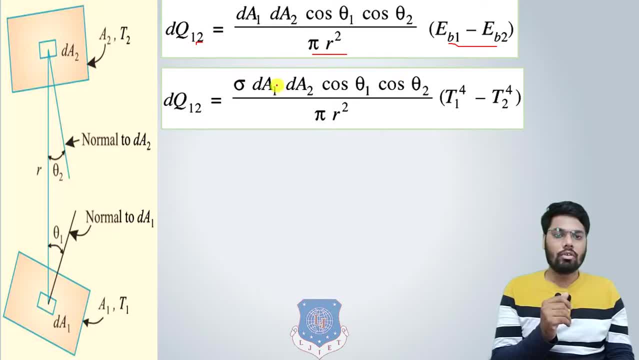 So sigma will be common. so it will be written out of the bracket. So in bracket it will be T1 raise to 4, minus T2 raise to 4.. So this equation represents net rate of heat transfer between surf dA1 and dA2.. 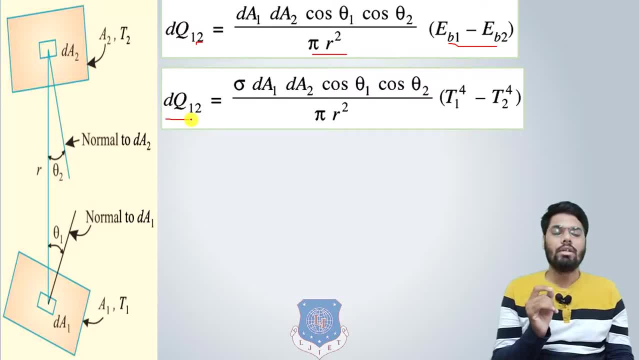 So it is represented by dq122.. This is the equation for differential area which we have considered from the old plane. We have considered dA1 from the total area A1,. we have considered dA2 from the total area A2.. 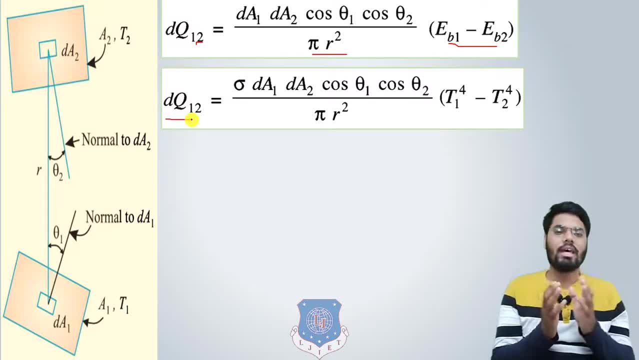 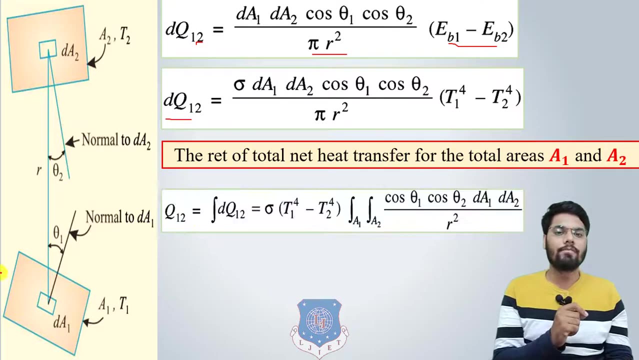 So if we want to apply this equation for the total area, we have to apply this equation for the total area A1. Then we need to integrate this equation with respect to total area A1 and A2.. So the rate of total net heat transfer for the total areas A1 and A2 can be written as: 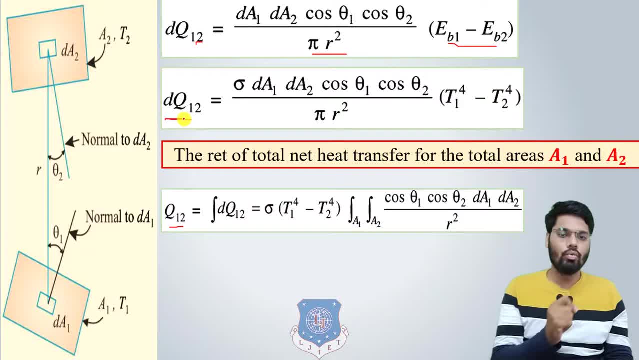 q122, here it is differential area, so dq122, here total area. so q122 is equal to integration of this. dq122 is equal to sigma T1. raise to 4 minus T2, raise to 4. integration with respect to total area A1 and A2.. 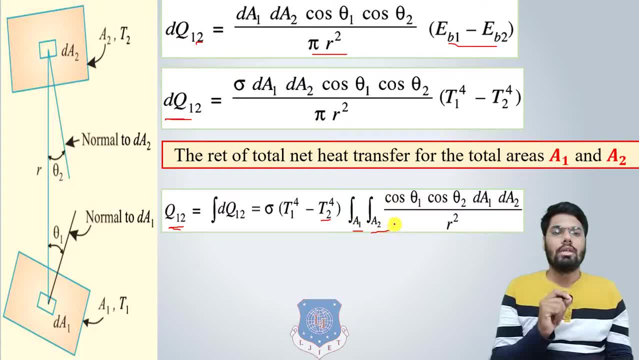 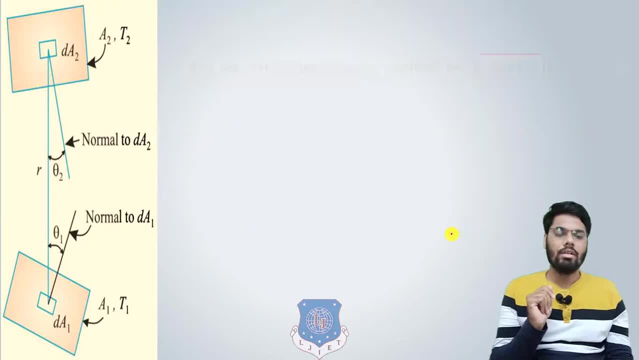 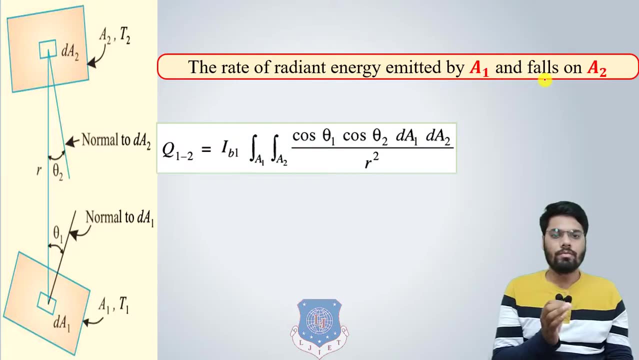 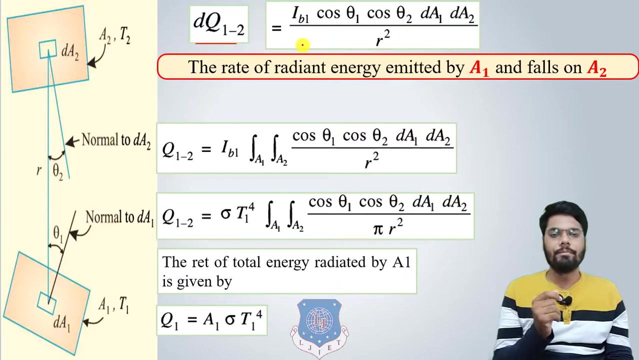 Cos theta 1, cos theta 2, dA1, dA2 divided by r square will remain as it is Now, the rate of radiant energy emitted by A1 and fall on A2, we have equation, this equation- we have seen this equation in our previous slide- that the amount of radiation. 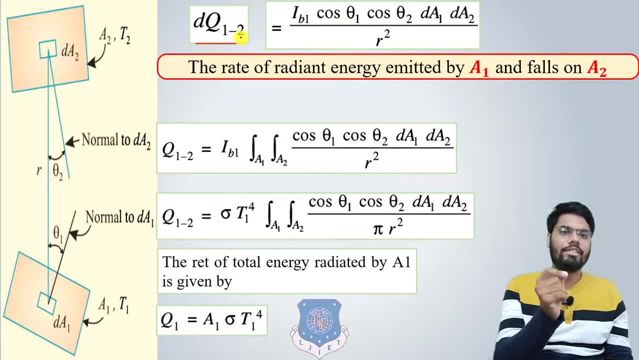 which is emitted by surface 1.. So from this equation we can write: this equation is for dA1 and dA2.. So for total area A1 and A2, we can write: q122, I b1, cos theta 1, cos theta 2, dA1, dA2,. 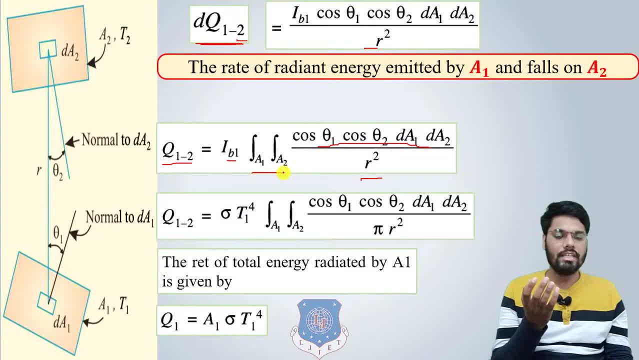 r square remain as it is For the total area. we have to integrate this equation by area A1 and A2.. Instead of I we can write down sigma T1: raise to 4 divided by pi. So this equation is for area A1 and A2.. 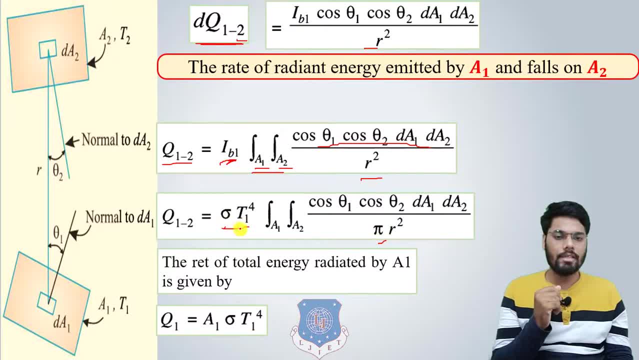 Instead of I b1, we can replace I b1 by sigma T1 raise to 4 divided by pi. So also the net rate of total energy which is radiated by A1 is given by again, I repeat again, the rate of total energy which is radiated by A1, total area of plate A, plate 1 is given. 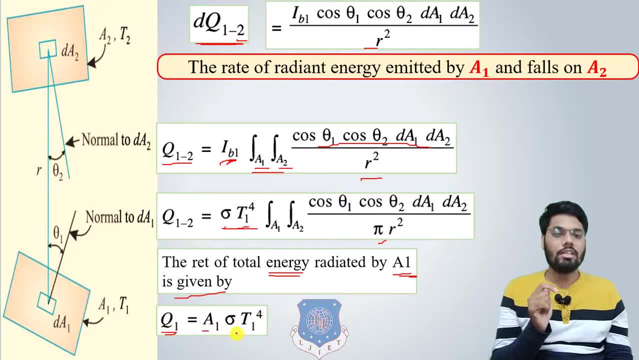 by q1 is equal to A1, into sigma T1 raise to 4.. This sigma T1 raise to 4 represents the emissive power And this A1 is the total area of the plate 1. So rate of total energy radiated means the amount of electromagnetic wave which is emitted. 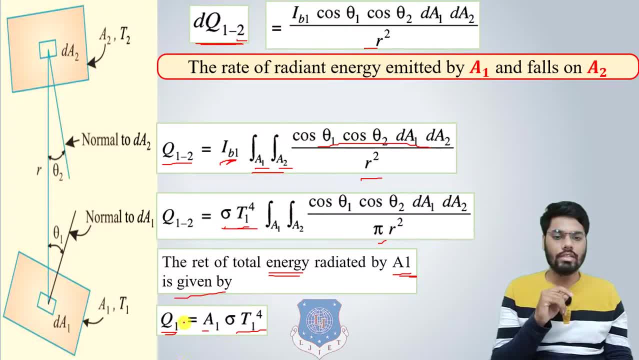 from the surface 1, from the plate 1 can be written as: q1 is equal to A1, sigma T1 raise to 4.. So this is: this equation shows the total amount of electromagnetic wave, or total amount of electromagnetic wave Or total amount of energy which is radiated by A1. 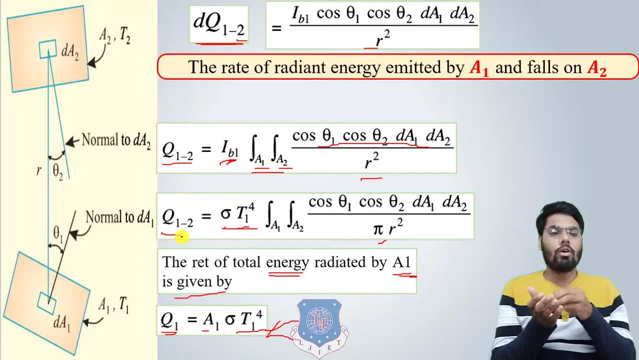 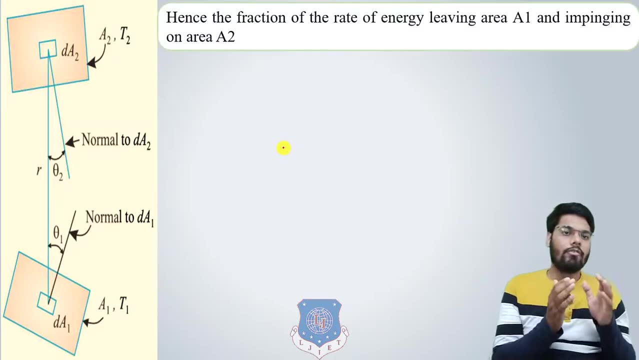 This q1 to 2 represents the amount of radiation, amount of energy which is absorbed by surface 2, which is emitted from surface 1.. So from these two equations we can write down the fraction of rate of energy that live in area A1 and incident or impinging on area A2 by q1 to 2 divided by q1.. 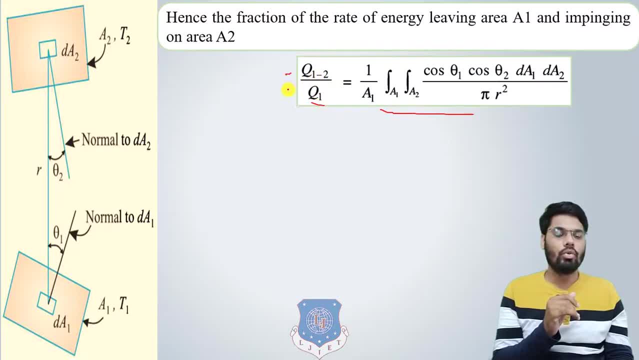 So we will get this equation by q1 to 2, divided by q1.. This q1 to 2 represent the amount of energy which is received by surface 2 from surface 1.. The net heat transfer between 1 to 2, the amount of electromagnetic wave which is emitted. 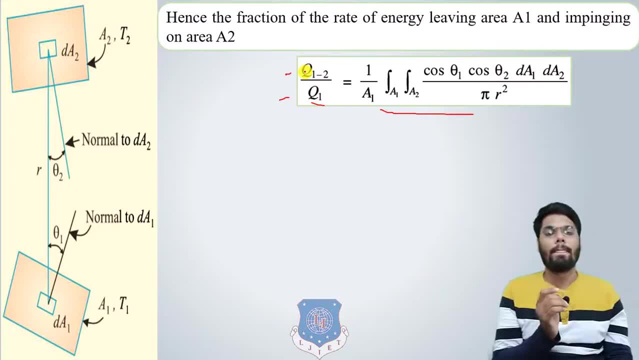 from surface 1 and incident on surface 2.. This q1 represent the total electromagnetic wave which emitted from surface 1.. So from that whole electromagnetic wave, only some amount of electromagnetic wave which is going to be incident on surface 2.. So the ratio of q1 to 2 divided by q1 is give us some value, which is the fraction. 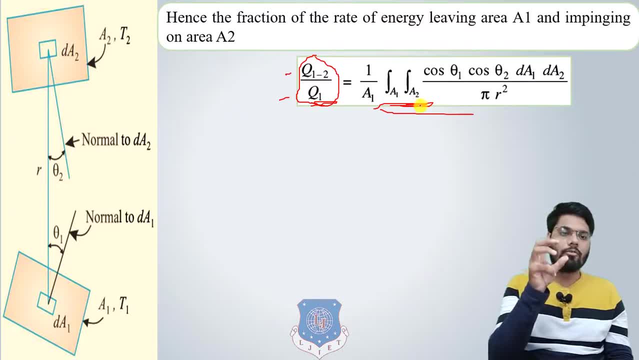 Fraction shows that this amount of electromagnetic wave is going to be incident on surface 2.. From total amount of electromagnetic wave which is emitted from surface 1.. So this q1 to 2 divided by q1, this equation is known- can written as f1 to 2, which represent 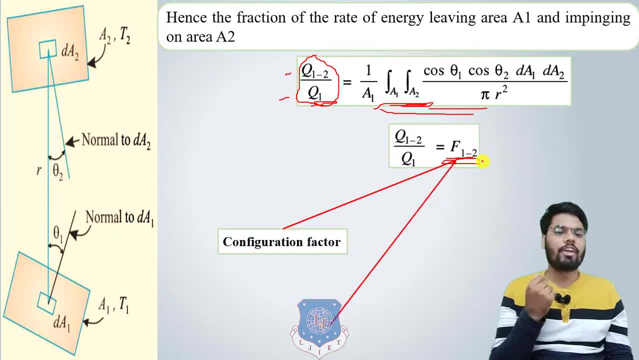 the fraction known as the configuration factor, or we can say that the surface factor written as the view factor, Because, according to orientation between surface 1 and surface 2, the amount of electromagnetic wave which is emitted from surface 1 and which is going to be absorbed by surface 2 can be. 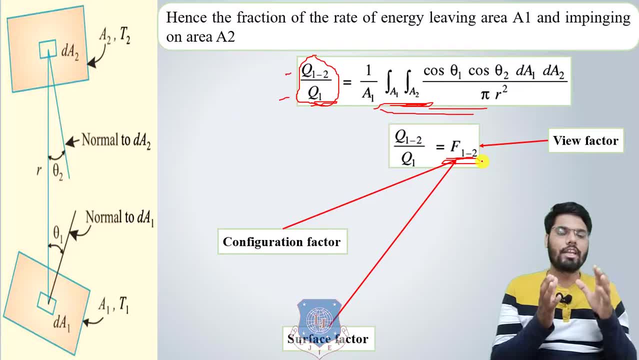 decided. So the in radiation mode of heat transfer orientation between two geometries plays an important role. So this f1 to 2, which is known as view factor, or configuration factor, or shape factor or surface factor, plays important role in heat transfer by radiation mode. 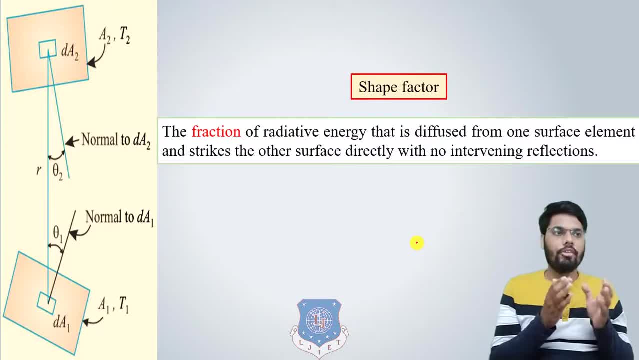 Now. so the definition of shape factor can be written as the fraction of radiating energy that is diffused from one surface. The Hybrid reaction times, corrector and acceleration can be known from this equation. We know: theyleft- sola, duty wave theballそれは. we have understood that the total amount of 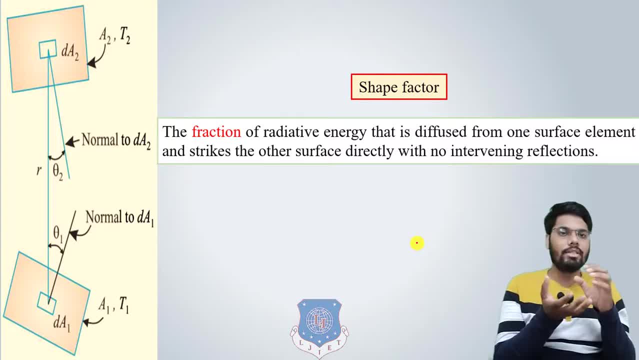 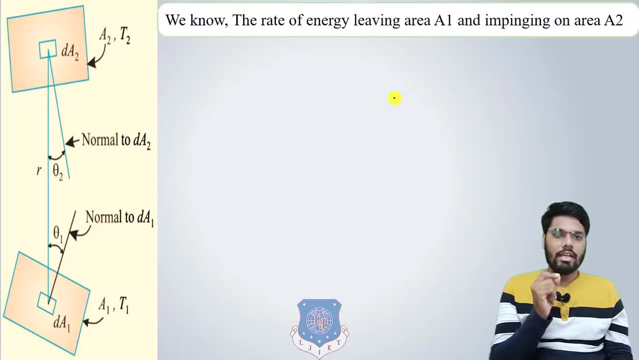 electromagnetic wave which is going to be emitted by surface 1, that total amount of electromagnetic is that from that total amount of electromagnetic wave, only some amount of electromagnetic wave is going to. the incident on surface 2, clear now we know that the rate of energy that leaving 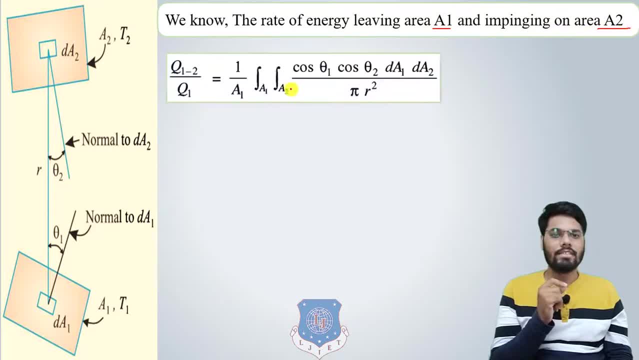 area A1 and incident on area A2 is Q1 to Q2 divided by Q1, this is our shape factor, or V factor. we also know it is denoted by F1 to 2, F1 to 2 means amount of electromagnetic. 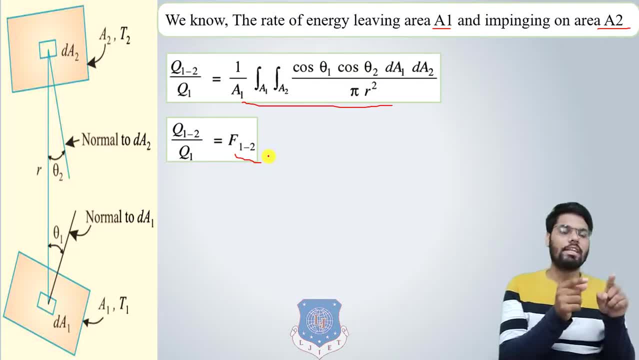 wave emitted from surface 1 and going to be incident on surface 2, we know the value of Q1, the total amount of electromagnetic wave or net energy this is going to be emitted by surface 1 is A1. into sigma T1 raise to 4, so from this equation, if we cross multiply, 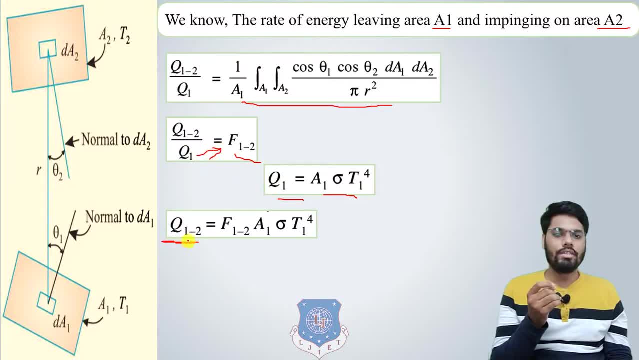 this Q1 with F1 to 2, we will get: Q1 to 2 is equal to F1 to 2. A1 sigma T1: raise to 4, so this F1 to 2 is equal to A1 sigma T1: raise to 4, so this F1 to 2 is equal to A1 sigma. 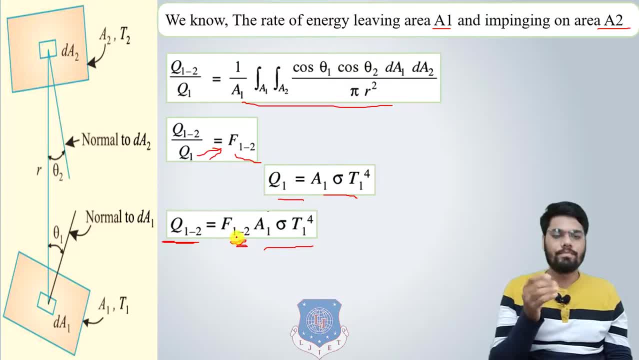 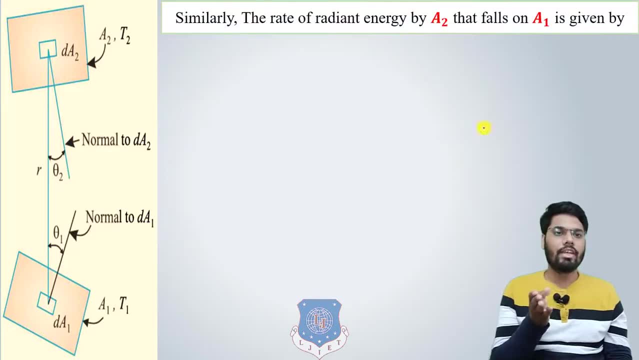 T1 raise to 4,. so this F1 to 2 is equal to A1 sigma T1 raise to 4,. so this is our shape factor, which is our fraction of Q1 to 2, so, as we have derived this equation for Q1 to, 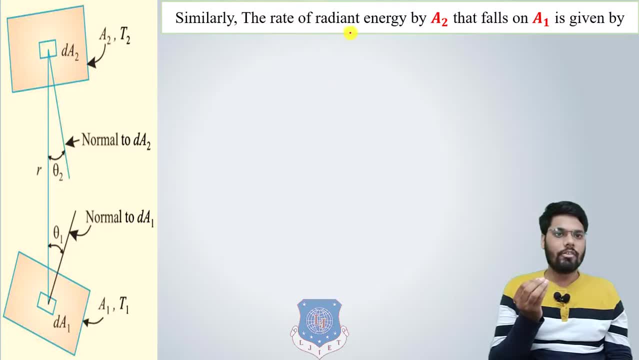 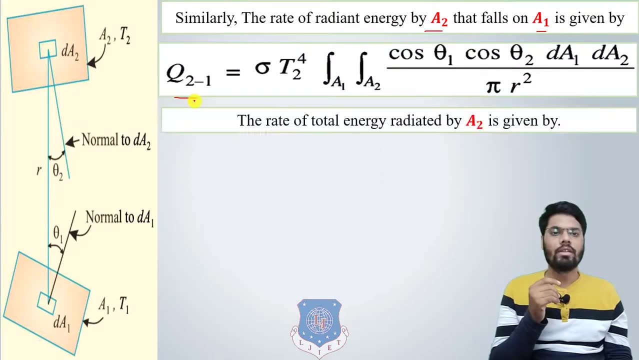 2. similarly we can write down the equation for the rate of radiant energy by A2 that falls on the area, so which is written as Q2 to 1,. here the rate of total energy A2 is given by Q2. A2 sigma T2 rise to 4,. similarly we can write down: Q2 to 1 divided by sigma. 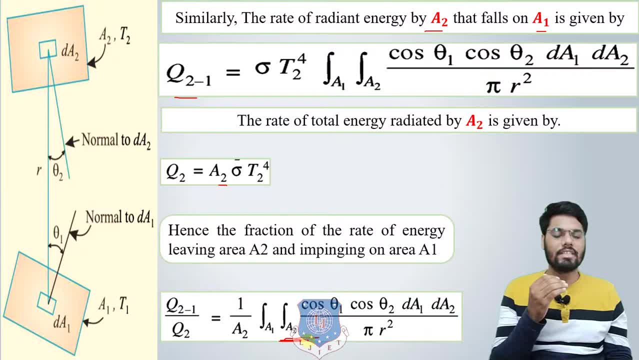 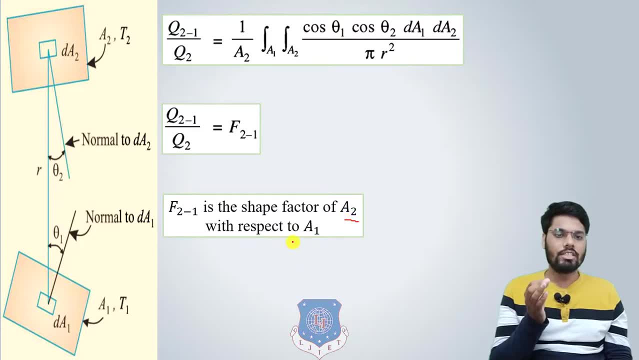 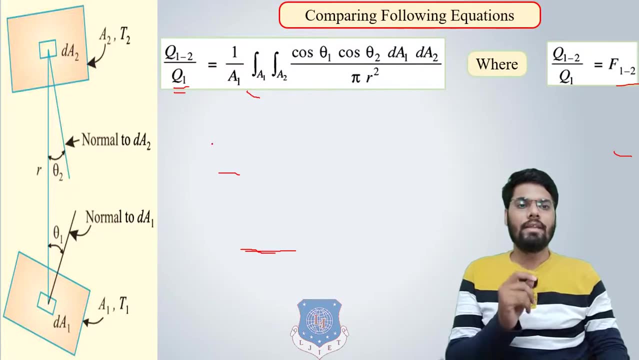 Q1 divided by Q2 and this equation represents F2 to 1, F2 to 1, which is shape factor of A2 with respect to A1.. Comparing the equations, first we have: Q1 to 2 divided by Q1 is equal. 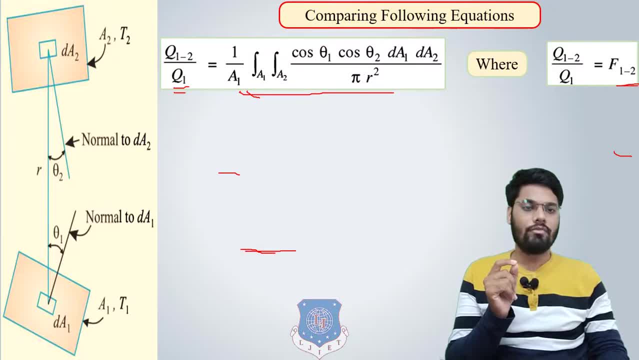 to this, where this whole term is known as the view factor or shape factor, which is divided by F1 to 2.. Similarly, for Q2 to 1, this is F2 to 1. this whole equation is known as the shape factor. By comparing these two equations, we will get A1. F1 to 2 is equal to A2, F2 to